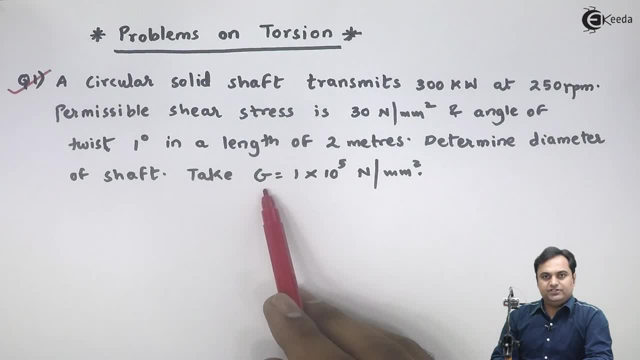 shaft. Take G, that is, modulus of rigidity is equal to 1 x 10, raise to 5 N·mm2.. This is the question which we have. Now let us write the data for this question Here. it is given that we have a circular solid shaft which transmits 300 kW, So power is given. 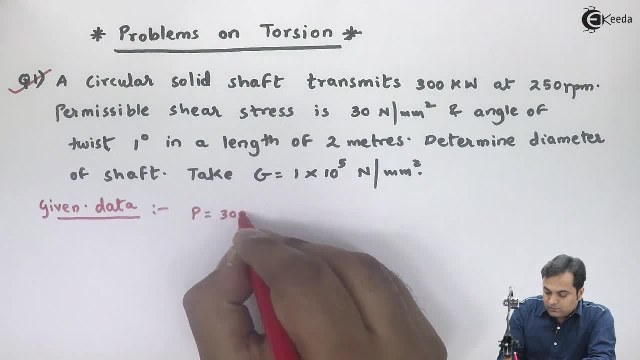 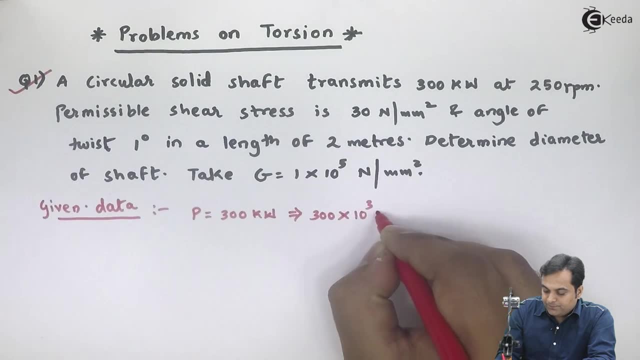 300 kW. So we have to convert it into watts. by multiplying it by 10 raise to 3.. RPM is 250.. So here I have: speed is equal to 250 rpm. Permissible shear stress is 30.. F is 30 N·mm2 and angle. 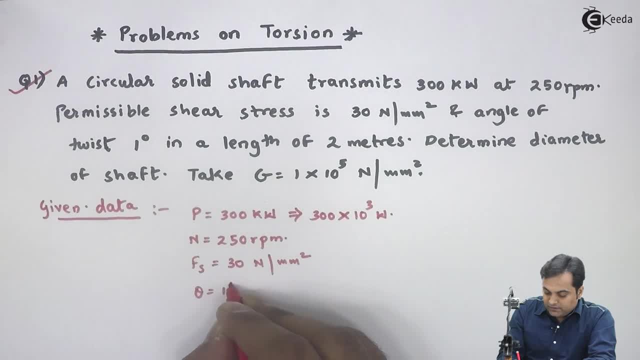 of twist is 1 degree, So theta is 1 degree. We can convert it into radians, So it is pi by 180 radian In a length of 2 m. the length is 2 m, which is equal to 2000 mm. Determine the diameter of shaft. So here we have to. 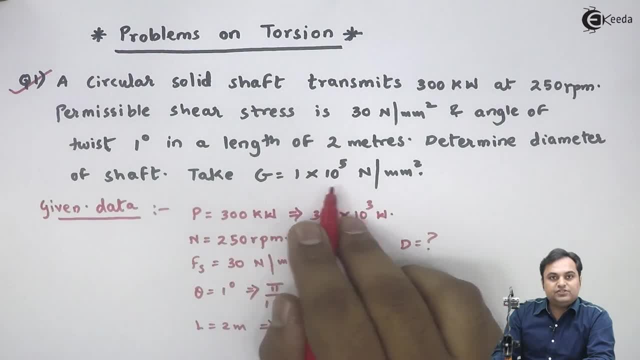 calculate how much is the diameter of the solid shaft. Take G is equal to modulus of rigidity: It is 1 x 10 raise to 5 N·mm2.. So here we have to calculate how much is the diameter of the solid shaft. Take G is equal to modulus of rigidity: It is 1 x 10 raise. 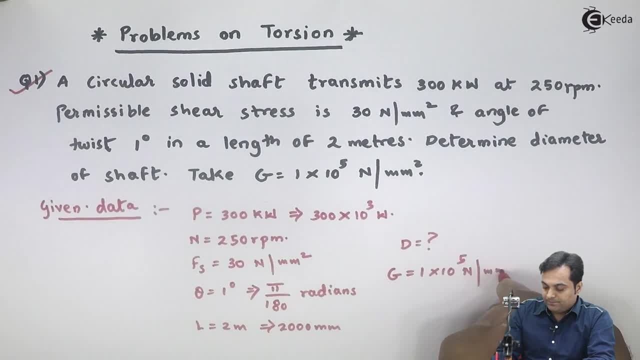 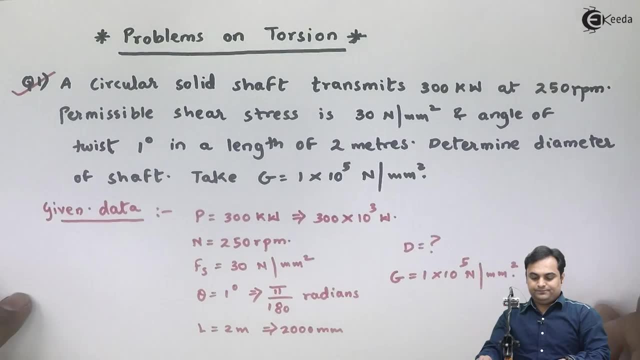 to 5 N·mm2.. So here we have to calculate how much is the diameter of the solid shaft? Take T is equal to 10, raise to 5 N· mm2.. So this is the question which we have. Now let us try to solve this problem, since in this question power is given. So I will. 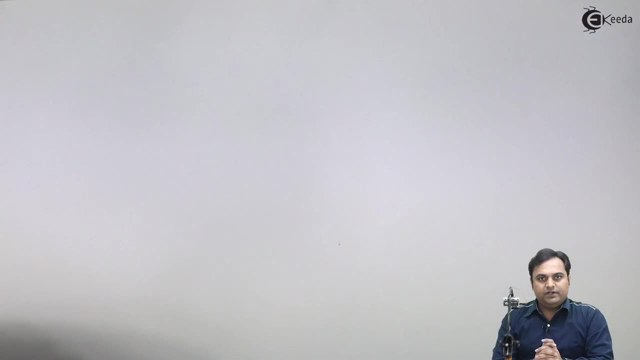 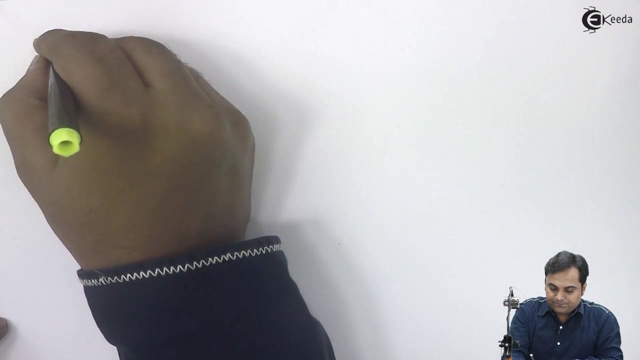 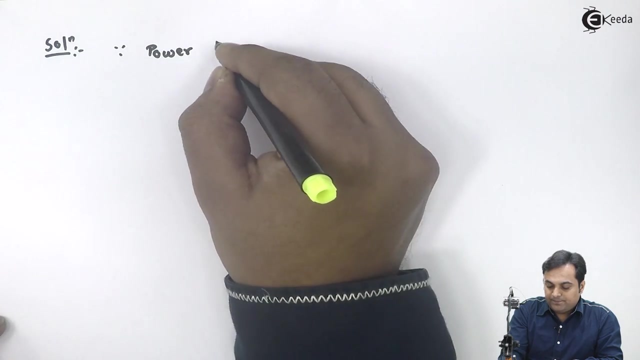 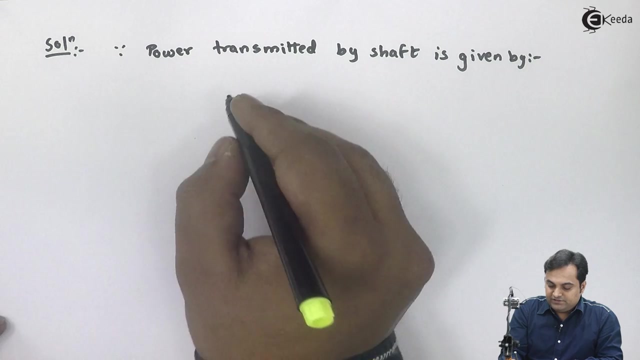 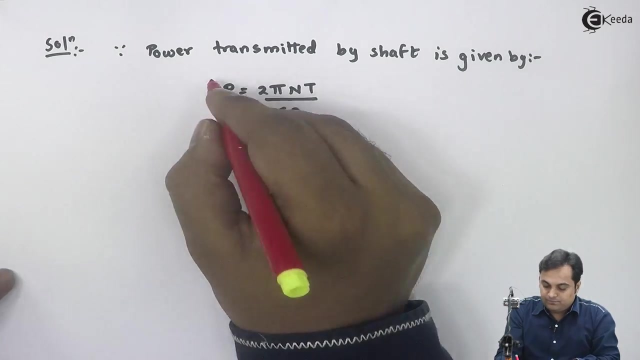 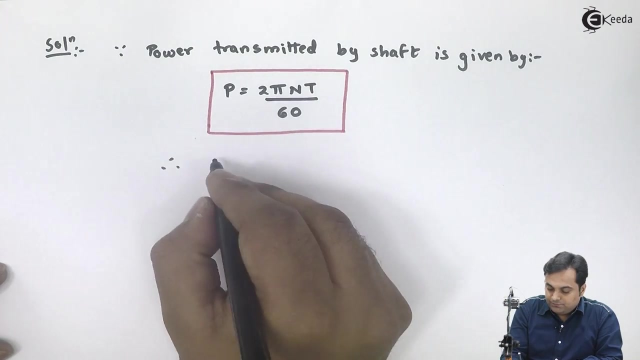 be using the equation of formula for power and try to get the torque value first. So let us write the formula. I will say that solution S radian N, since power transmitted by shaft is given by The formula, is: p is equal to 2 pi nt upon 60. therefore, t is equal to p into 60 divided. 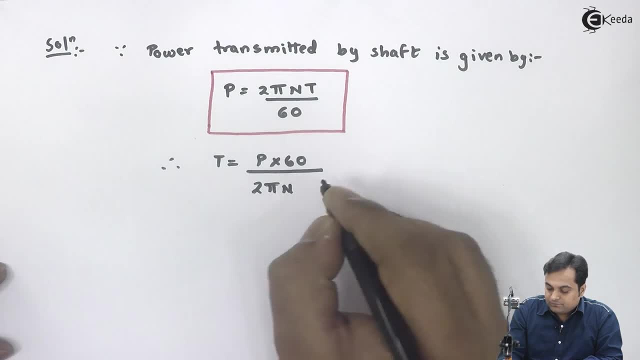 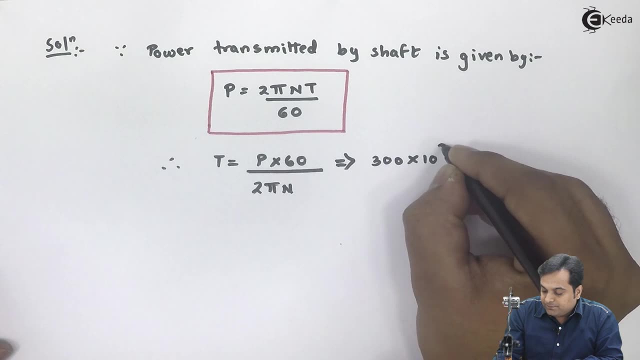 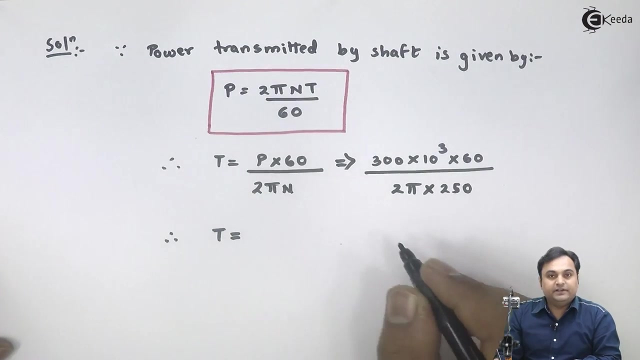 by 2 pi n, power is given as 300.. into 10 raise to 3, into 60, divided by 2 pi into n, which is 250. so if I calculate here, I will be getting the value of torque, which comes out to be 11.46. into 10 raise to 3 newton. meter Which I can connect to the power transmitted by the shaft. So I will be getting the value of torque, which comes out to be 11.46, into 10 raise to 3 newton meter which I can connect to the power transmitted by shaft. 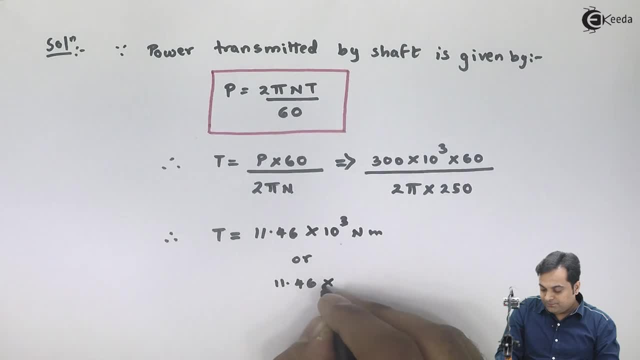 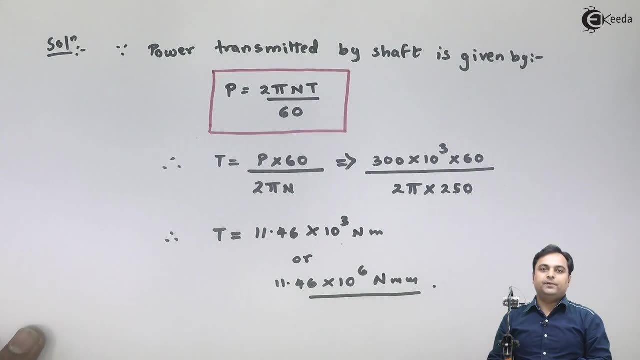 which I can connect to the power transmitted by the shaft, Which I can connect to the power transmitted by shaft. This is the value of torque which I am getting. The problem is, I have to calculate the diameter of solid shaft. So for that I will be using two criteria". 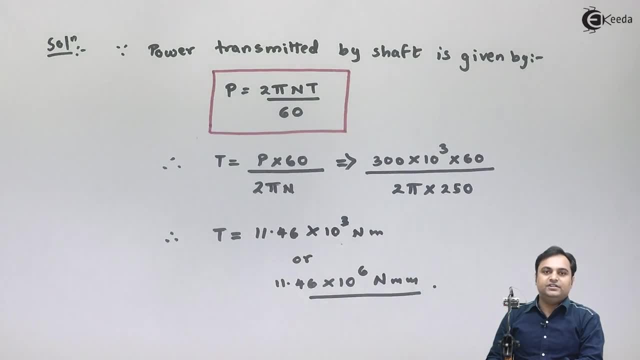 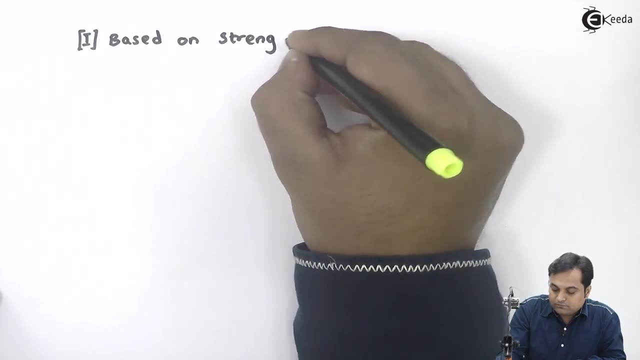 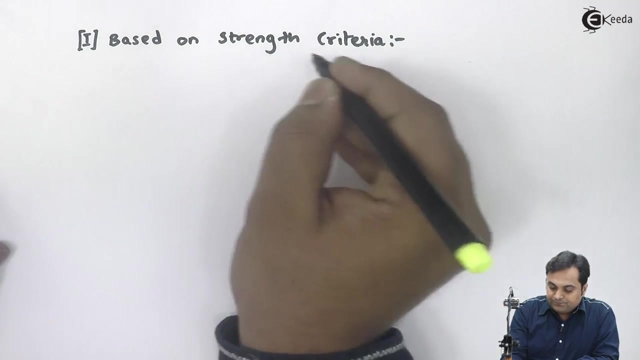 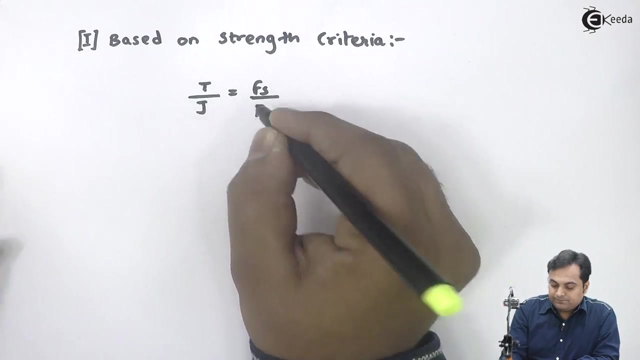 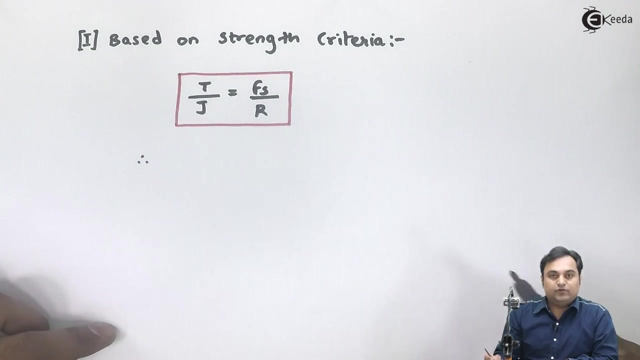 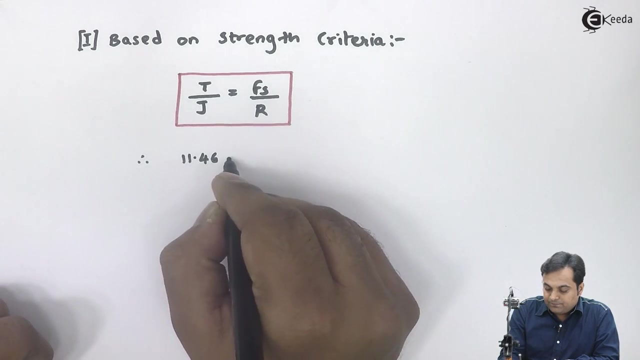 First strength criteria and the second one rigidity criteria. So we take the strength criteria. So, based on strength criteria, we know the equation is given: by T upon J is equal to Fs, by R, therefore T value- we have just now calculated it is 11.46 into 10, raise to 6. 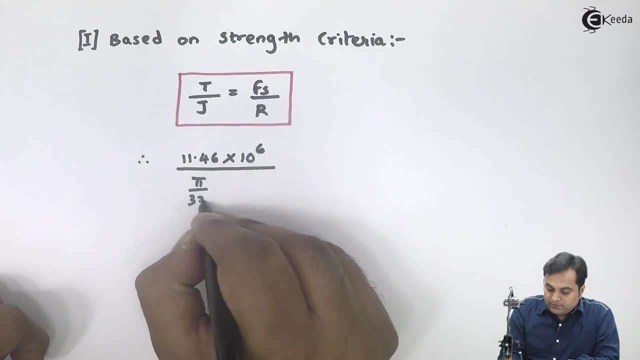 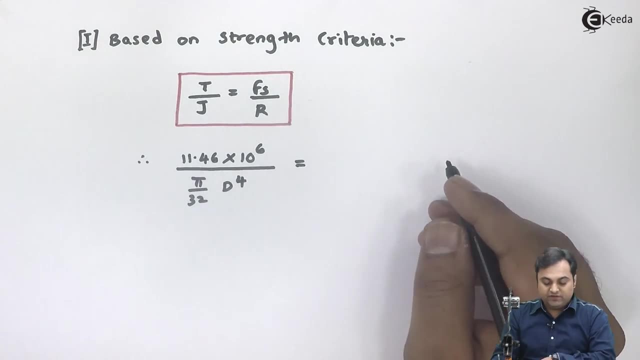 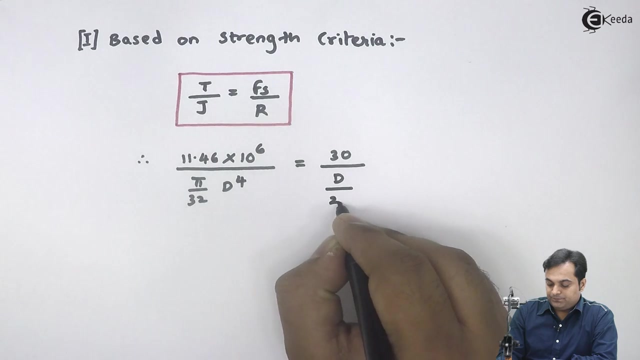 J is pi by 32. diameter raise to 4 for solid shaft Fs Shear stress is given in the problem as 30 and R is equal to diameter divided by 2.. So here, if we see from left hand side and right hand side, D and D will get cancelled. 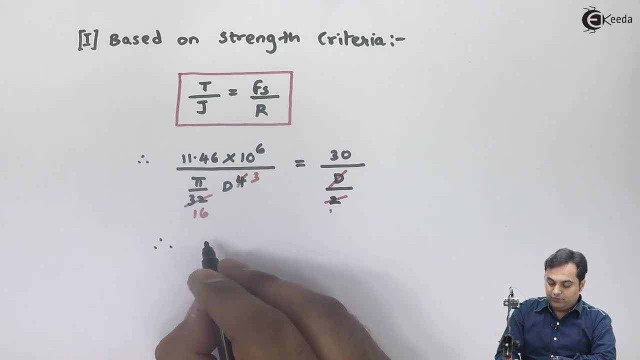 So here I can write this: as, therefore, D cube will be equal to this, D cube shifts on the other side And 30 will come into the denominator. So here I have 11.46 into 10, raise to 6, divided by pi, by 16 into 30.. 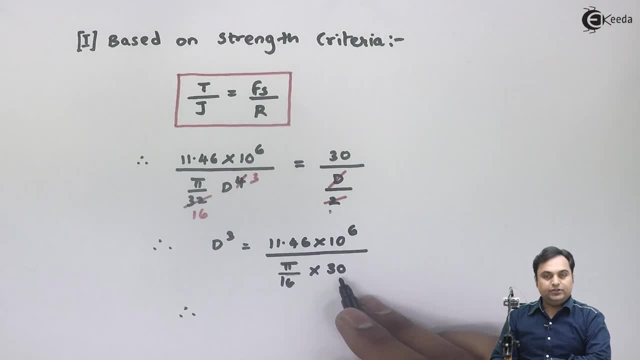 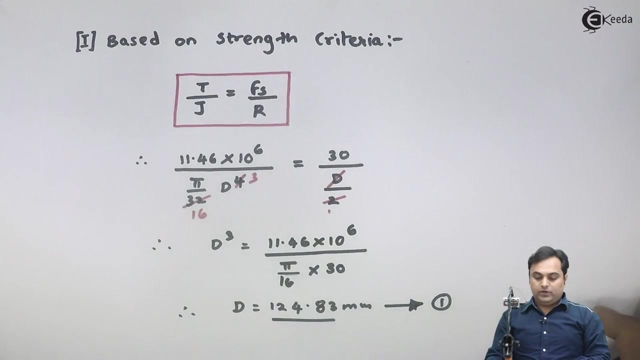 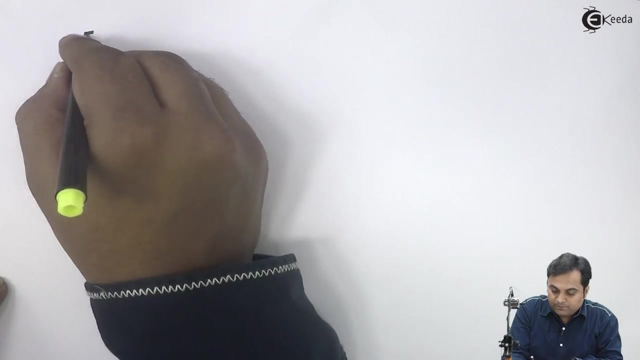 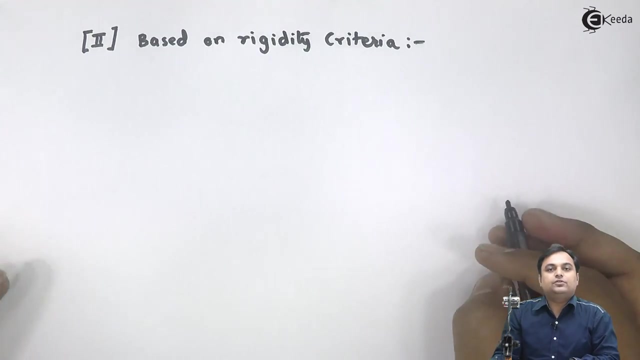 So from this, if I calculate numerator upon denominator and take the cube root of the answer, I would be getting D, which comes out to be 124.83.. Now here it just comes to 10 Hữa, And I will take thisresses fella m. 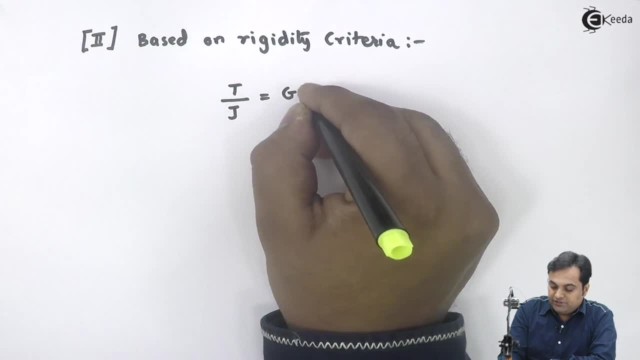 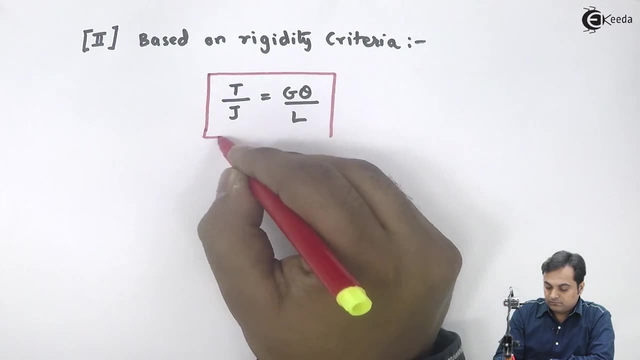 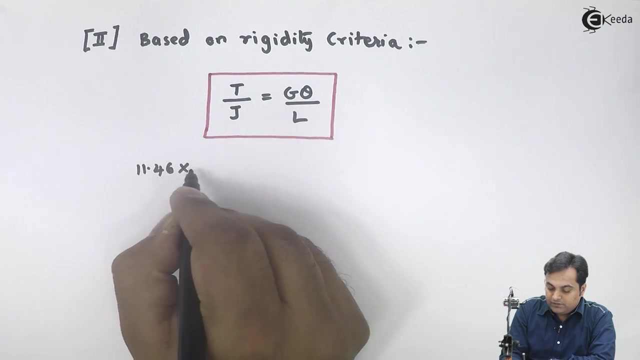 I will cod this as my equation number 1.. Now, as I have used strength criteria, Now I will be using the rigidity criteria. by L, the value of T, it is eleven point four, six into ten, raise to six, J is pi. 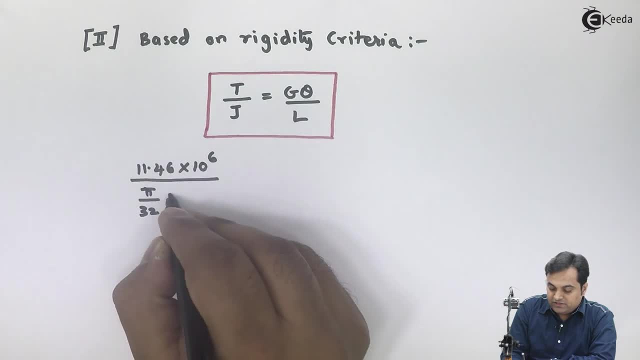 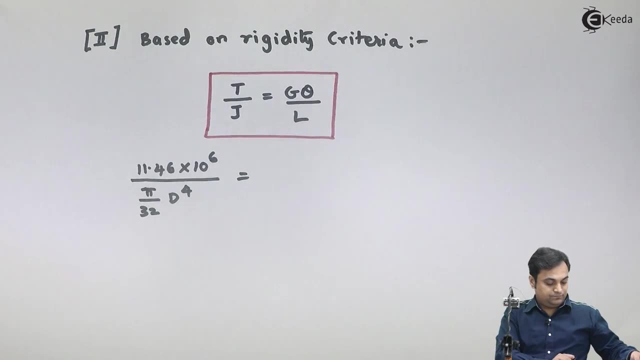 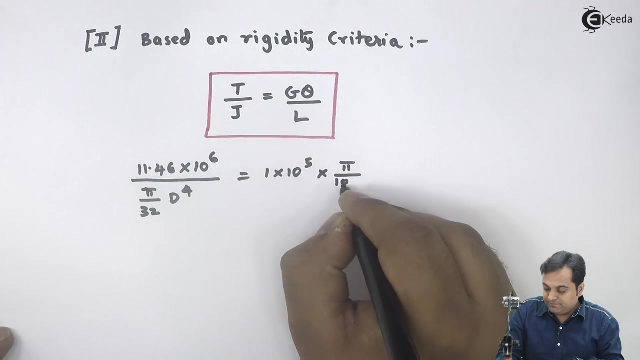 by thirty two, D raise to four. for solid shaft, the value of G is given in the question. G is 1 into 10 raise to 5. theta is 1 degree. so it is pi by 180 radian divided by the length of shaft, which is 2000 mm. so from this, if I calculate all, 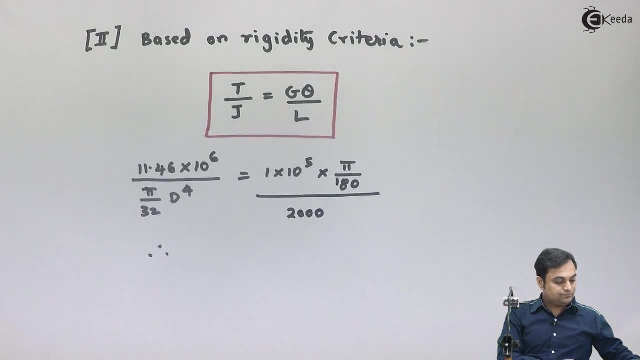 the terms. first I would be getting D raise to 4 answer. the value of D raise to 4 comes out to be: it is 13.097 into 10 raise to 6, and if I take the square root twice, I will be getting the answer of D, which in this case it is 107.5 mm. 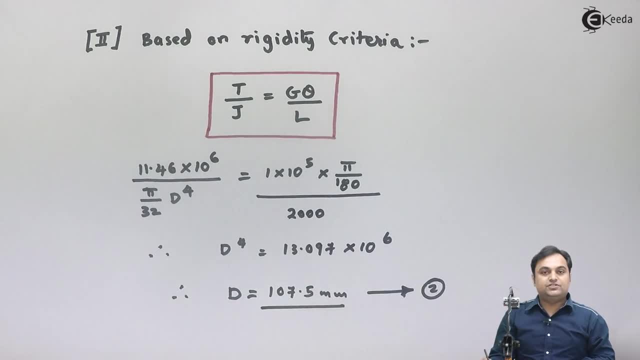 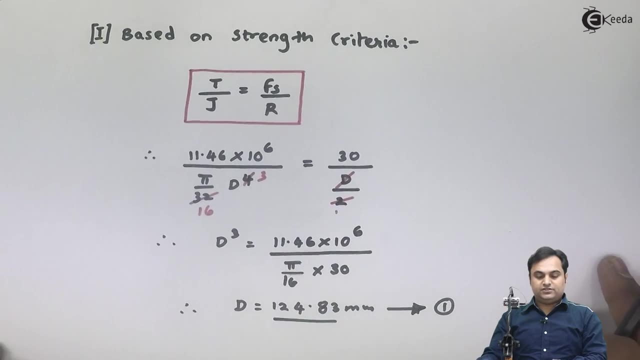 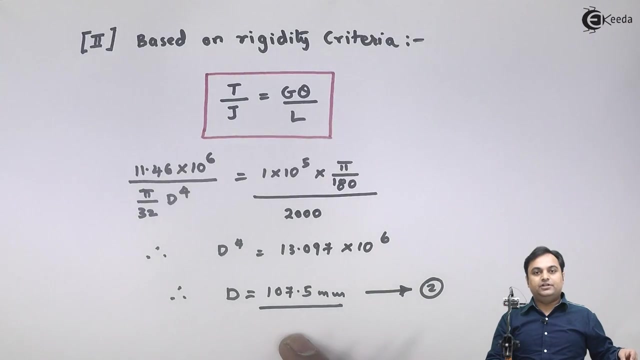 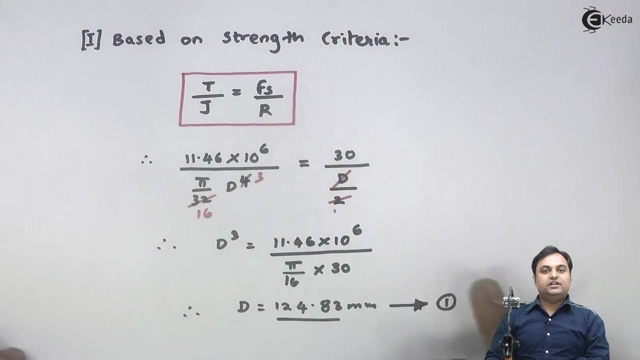 I will call this as my second equation. now, if I compare equation number one, in which the diameter was 124.83 mm, equation number two, in which the diameter is 107.5 mm. so out of this I am getting the diameter by strength criteria as more, so we have to select the greater diameter, because if we are